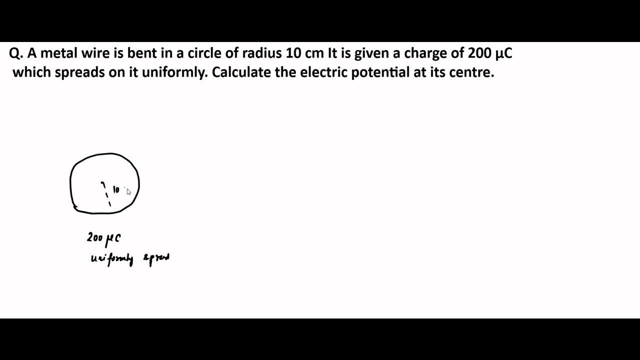 We have to find the electric potential at the center, which is 10 centimeter away from it. So here what we will do is that we will kind of divide each of these- you know, this metallic circle- into small, equal segments, each having a charge of dq, And each of these segments 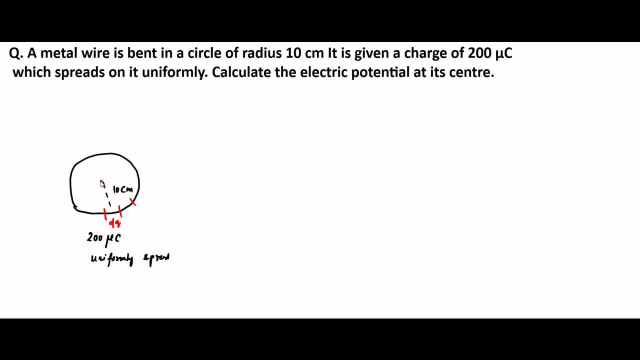 each dq segment, small segment will contribute to a small potential dv and considering all of these segments of equal values dq, they will all contribute their potential dv which will get added together. sum together so here the electric potential dv contributed because of a small charge segment dq is equal to 1 by 4 pi epsilon, 0 dq by r. okay, so the total potential is equal to. 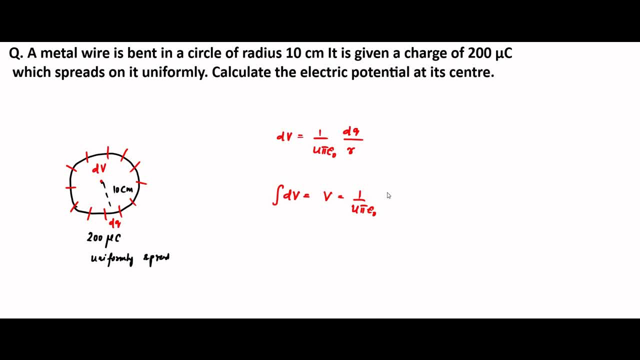 1 by 4 pi, epsilon, 0 cube by r. okay, which is the total charge. now we are given that the total charge, which is spread uniformly, that is equal to 200 microcoulomb. so the potential at the center due to this total charge which is spread uniformly, that is equal to 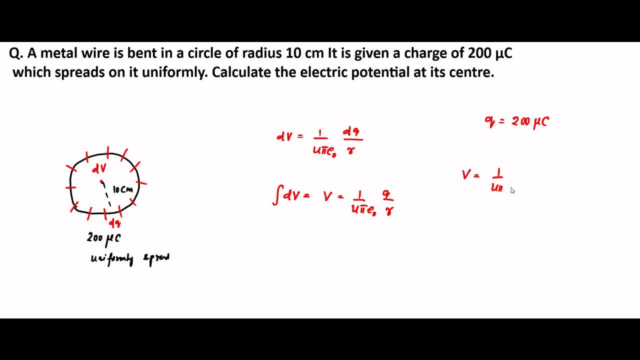 1 by 4 pi, epsilon, 0, 200 microcoulomb, that is, 200 into 10, to the power minus 6 by r, which is equal to 10 centimeter, okay, equal to 10 to 10, to the power minus 2 meters. 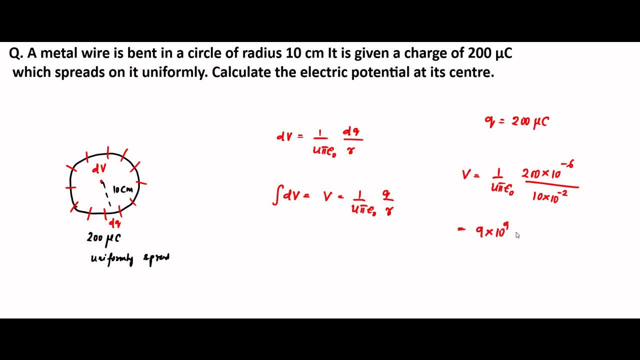 so is equal to 9 into 10, to the power 9, that is, 1 by 4 pi. epsilon 0 into 200 microcoulomb into 10, to the power minus 6, by 10 into 10, to the power minus 2, converting it into meters. 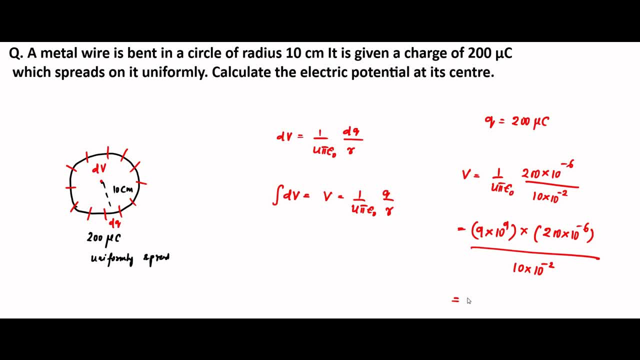 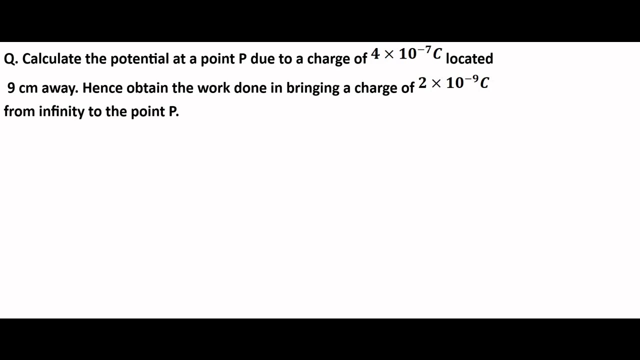 so the result is coming 18 into 10 to the power 6 foot. that is the potential at the center, okay, center of the metallic cell. okay, so here is another question. it is given to calculate the electric potential at a point p due to a charge of 4 into 10 to the power minus 7 coulomb located 9 centimeter away. okay, 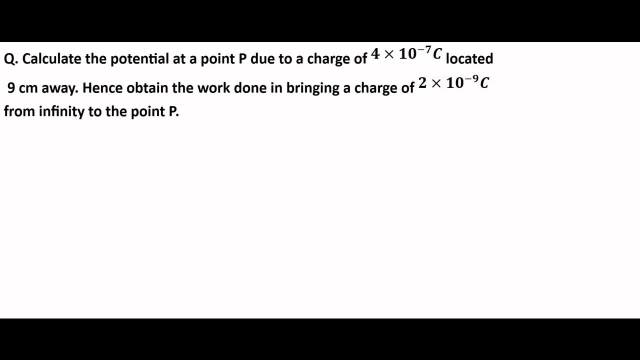 and then we have to find out the work done in bringing a charge of 2 into 10 power X笑 9m by r from x n the point P: ok. So here the situation is: we have a charge. ok, we have a charge, we will. 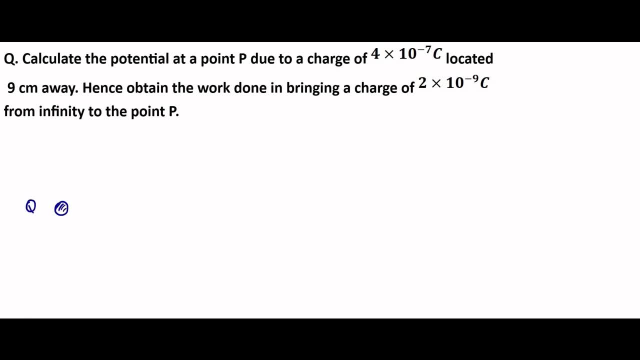 call it. let us say source charge. ok, source charge, that is a. it has a value of 4 into 10 to the power, minus 7 coulomb. ok, and we have to find the electric potential at a point P which is 9 centimeter away from it. ok, So here the electric potential at point P is: 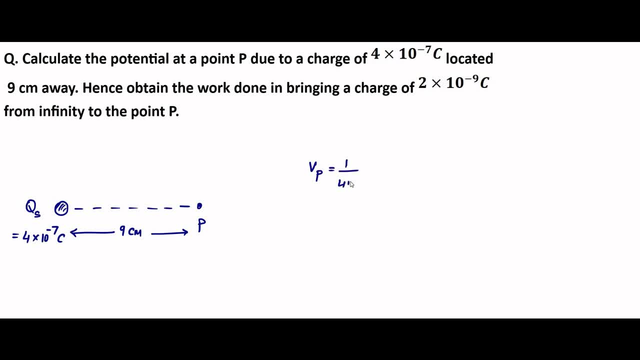 equal to 1 by 4 pi, 4 pi epsilon 0, source charge Q, s. by this distance r, which is equal to 9 into 10, to the power 9 into 4 into 10, to the power minus 7, by 9 into 10, to the power minus 2 meters. It is in centimeters. 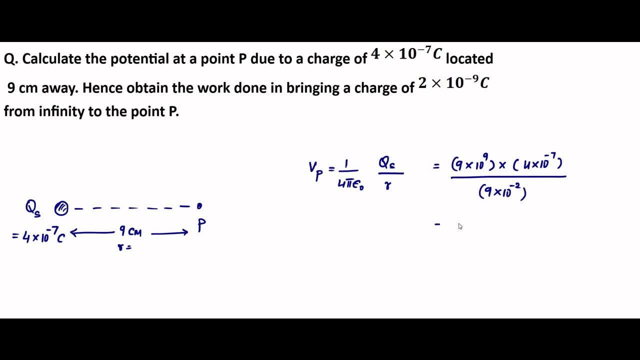 so always convert into meters. So this electric potential, that is coming 4 into 10 to the power, 4 volt. Okay, the electric potential at point P. Now, if you remember, we have already discussed electric potential. electric potential, energy Suppose in an electric field. we have to move. 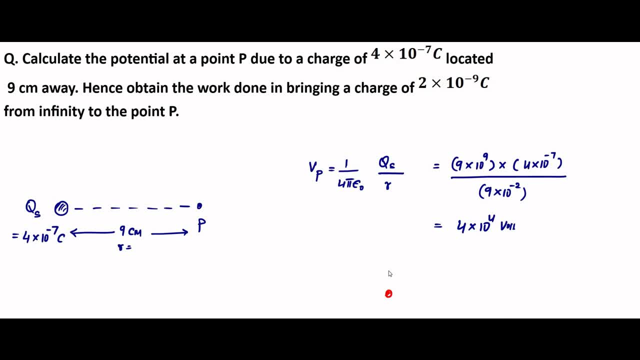 a charge from an initial point- let us say I- to a final point. let us say F. Okay, initial point to final point, if you want to do the work. So the work done in moving the charge from the initial point I to final point F is equal to the value of the charge. let us say we: 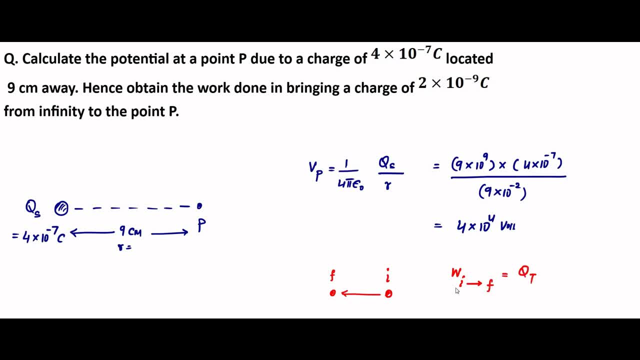 are considering a test charge Q t. we are moving it from I to F. work done in moving the test charge from I to F. that is equal to the value of the test charge multiplied with the difference of the electric potential between the final point and the initial point. Okay, work done. 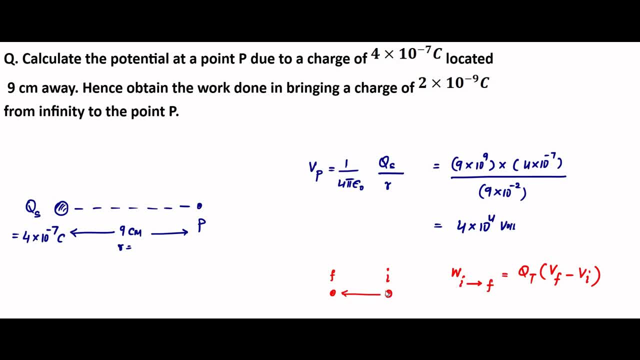 in moving a test charge Q t from point I to F, that is equal to the value of the test charge multiplied with the difference of the electric potential between the two points: V F minus V I, final point potential minus initial point potential. So here let us say, let us say: 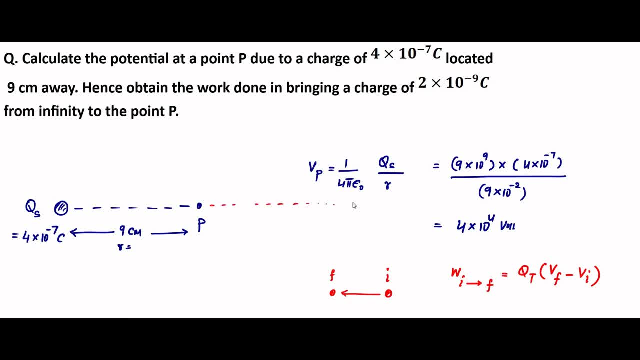 we have a test charge which is located at infinity, far away, the potential at infinity that is equal to zero volt. we are moving a test charge, let us say Q, t, which is equal to 2, into 10, to the power minus 9 coulomb, from infinity to this point. we have already.